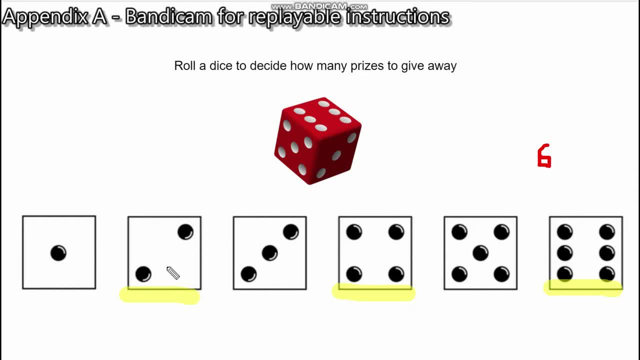 Okay, But how many even numbers are there? One, two, three, So a three Three out of six chance, which is actually half. You see there's three odd numbers and three even numbers, which means there's a 50-50 chance Mrs Leopard will roll an even number. 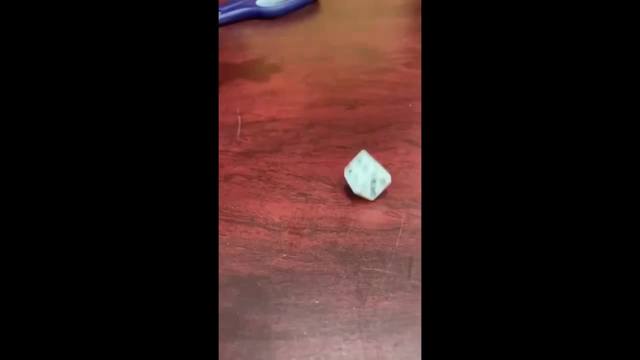 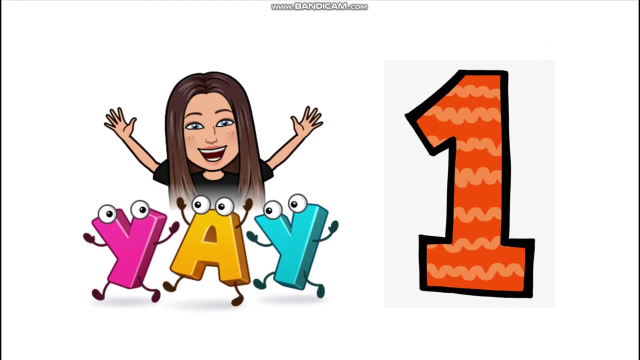 Let's see what Mrs Leopard rolls. Now Mrs Leopard knows that she's going to give out one prize because she rolled a one on the dice, But who should get the prize? Is there a fair way to decide Who can get the prize? 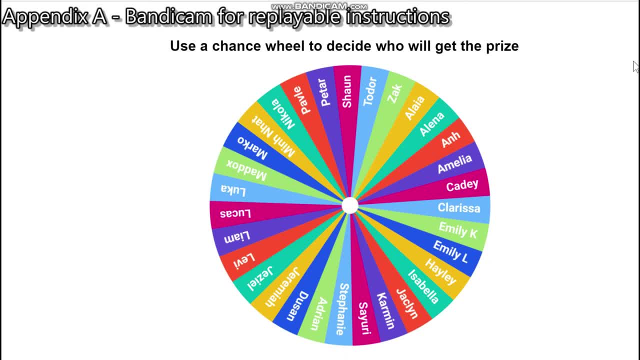 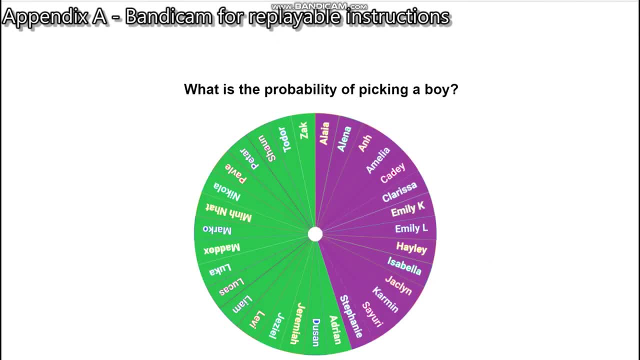 What she does is she puts all of the people in 3-4-T in a chance wheel, But before she spins the wheel she asks some questions Like: what is the possibility of picking a boy? She colours in all of the boys' names green and all of the girls' names purple. 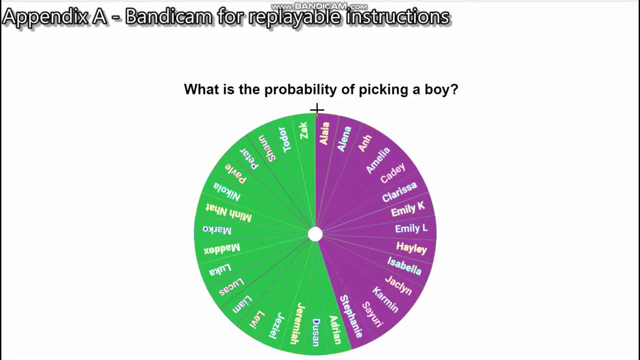 She notices that if she draws a line straight down the middle, she's going to get the prize. We would be able to find out where half is. The boys have more than half of the circle coloured in, which means that they are more likely to be picked than a girl is. 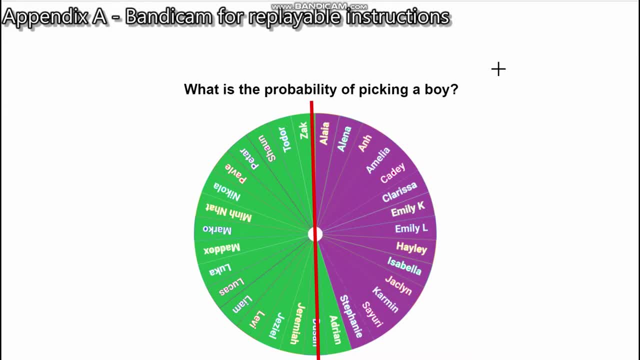 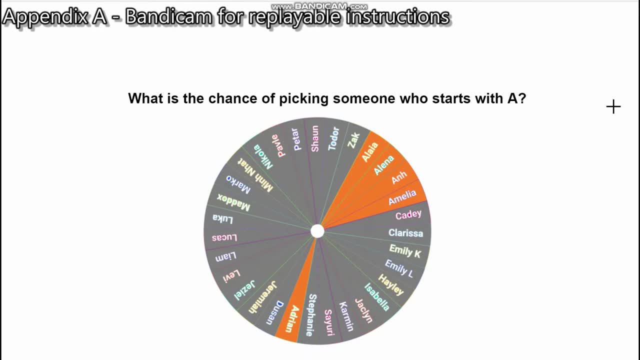 because there are more boys on the wheel than there are girls. The next question she asks is: what is the chance of picking someone who starts with A? She colours in all of the people who start with A in orange and everyone else in grey. 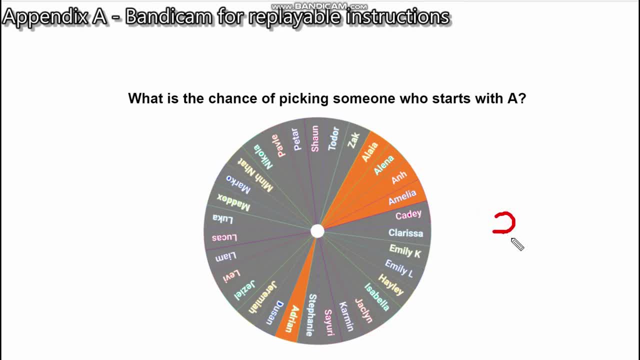 There are 31 students in the class, 31 total students if you count up all of the names, And there are only 1,, 2,, 3, 4, 5 students who start with A. This is not many students. 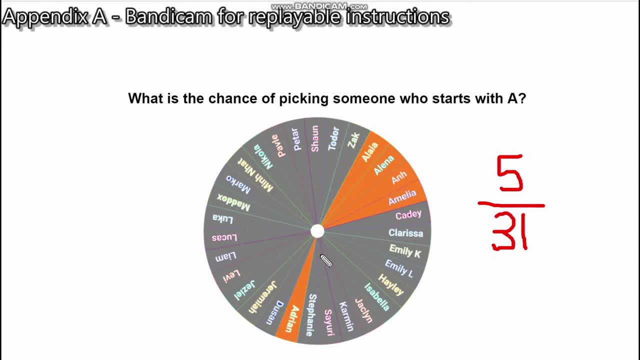 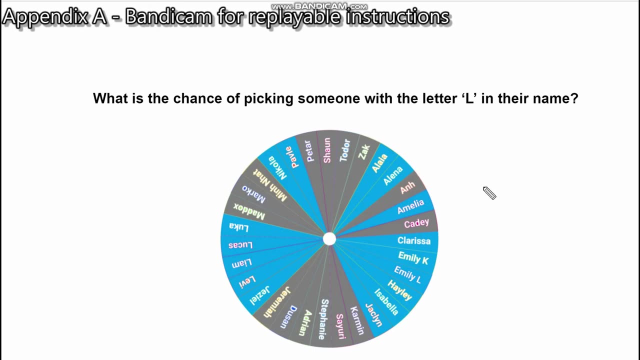 If you look at all of the grey, there's not that many orange students. So we're going to say this is very unlikely. What is the chance of picking someone with the letter L somewhere in their name When she knows that there are a total of 31 students in the class? 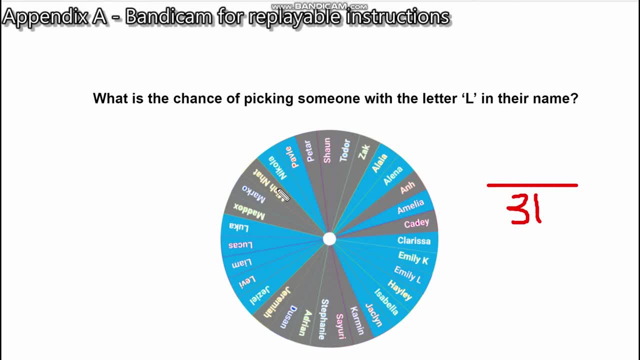 so she's going to put that figure down here And there are 1,, 2,, 3,, 4,, 5,, 6,, 7,, 8,, 9,, 10,, 11,, 12,, 13,, 14,, 15, 16.. 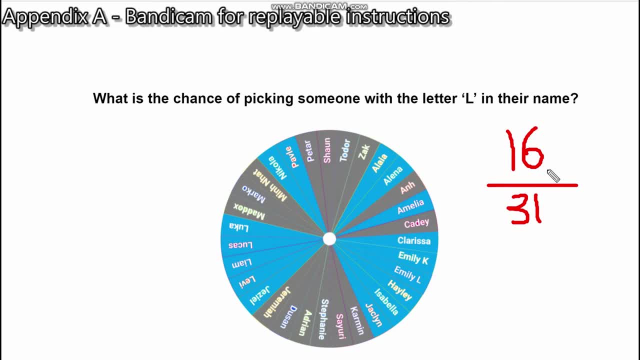 people with the letter L in their name. Half of 31 is 15.5.. But you can't really have a half of a person, which is what 0.5 means. So we can round that up to 16.. 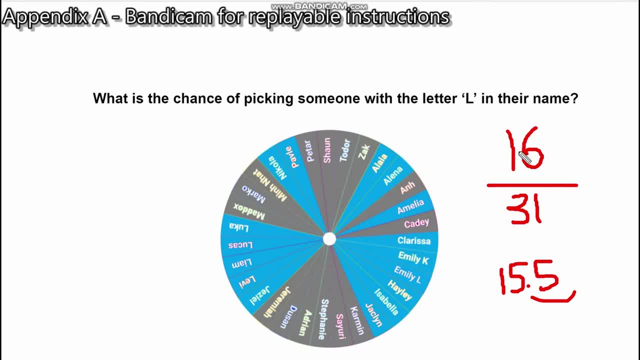 So about half of the students in 3.4T have an L in their name. It is equally likely that the person that is picked will have an L in their name or won't have an L in their name, So it is equally likely. 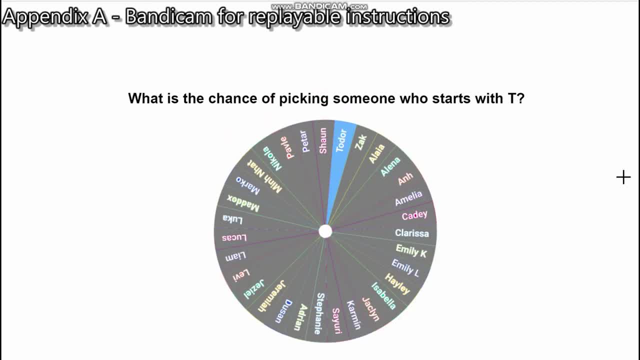 The final question she asked is: what is the chance of picking someone who starts with T? Well, there's only one person in the class that starts with T, and it's Toddy. She remembers that there's 31 kids in the class. 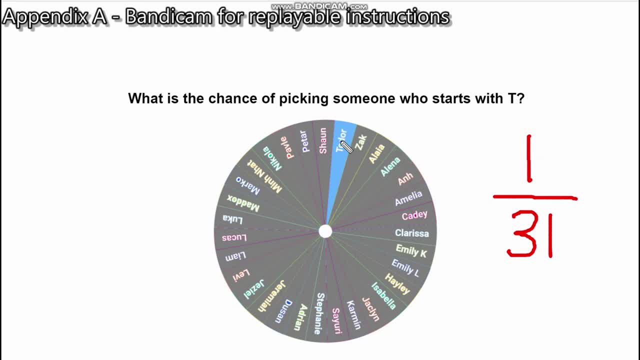 but only one student that starts with T, So actually it's the very least likely pick. It is more likely that the person picked will start with any other letter, So starting with T is least likely, OK, so who's the winner? 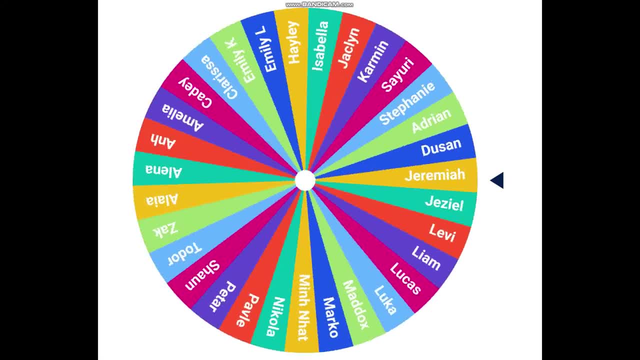 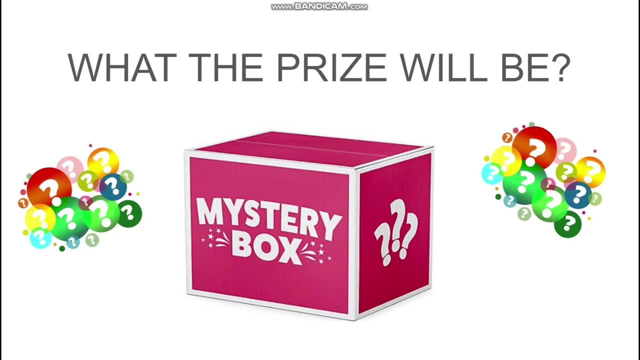 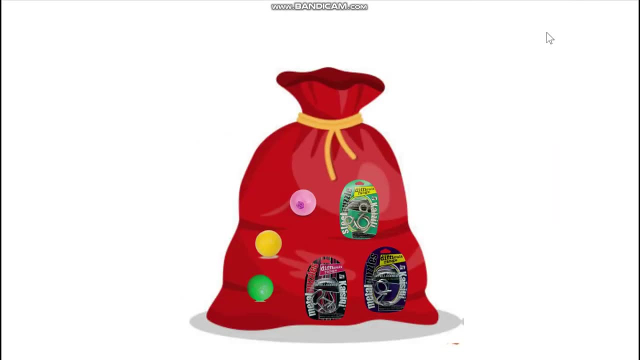 Let's spin the wheel and find out. And Sayuri is the winner of the prize. Hang on a minute. We still don't know what the prize will be. What is Mrs Leopard going to do to decide? She finds her trusty prize bag and puts her hand in. 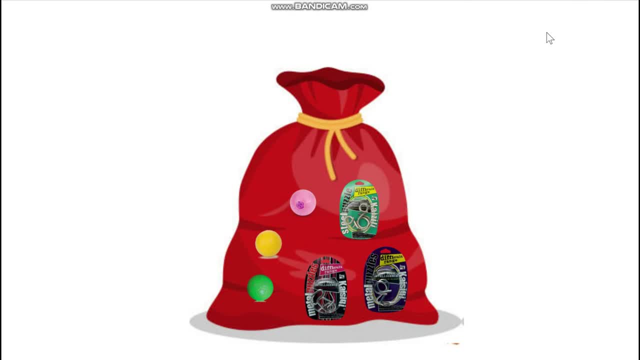 What is the probability- that's another fancy word for chance- of Mrs Leopard picking up a Kaizili puzzle? First let's look at all of the possible outcomes. We've got one, two, three, four, five, six possible outcomes. 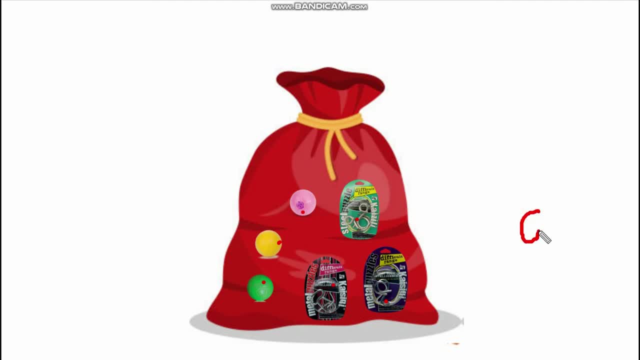 because there are six prizes in the bag, So let's put down six. But we want to find out what's the probability of Mrs Leopard picking up a Kaizili puzzle. How many Kaizili puzzles are there? One, two, three.